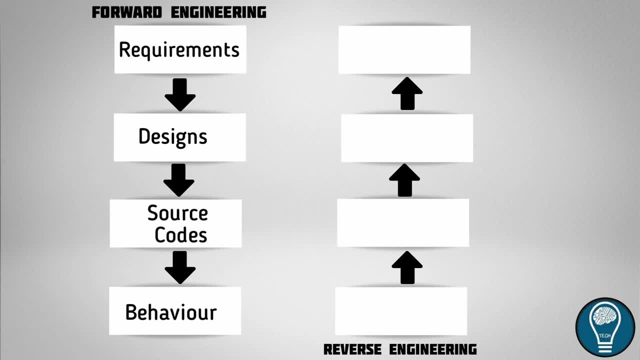 we use aria-b: the development of the base model. This is the first step, followed by the development of the model, Reverse engineering. it goes up from bottom: Behavior, source code, designs and requirements. Let's see the waterfall model of software development. 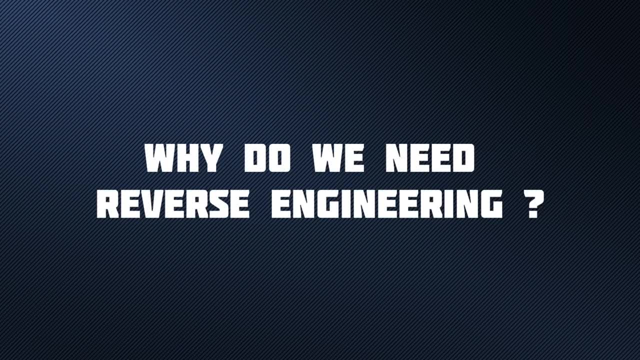 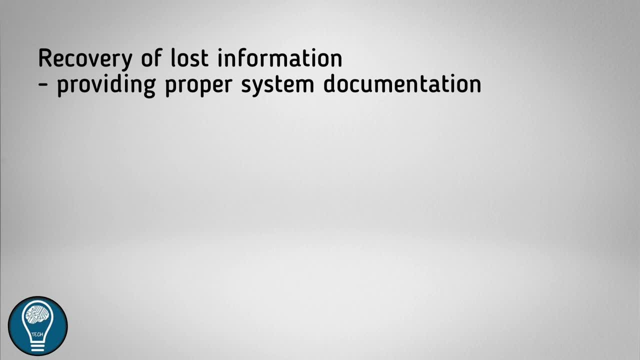 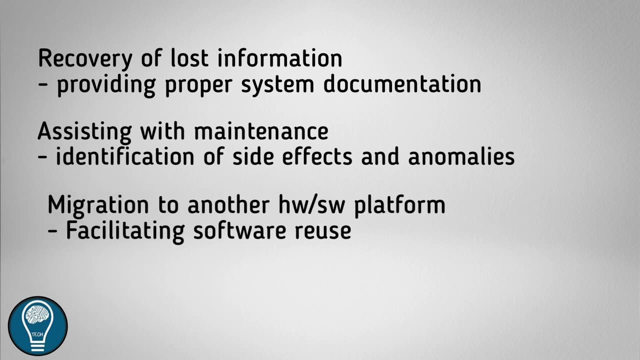 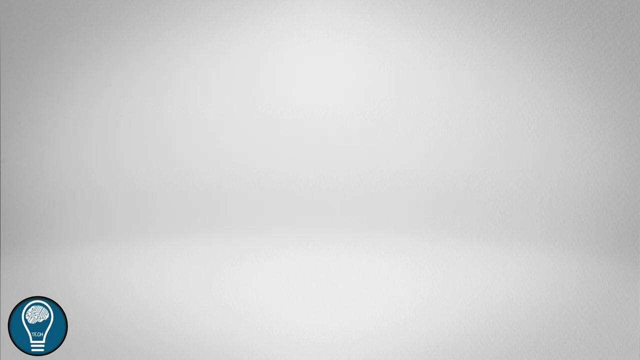 You might think. why do we need reverse engineering? Recovery of lost information, Providing proper system documentation, Assisting with maintenance, Identification of side effects and anomalies, Migration to another HW-SW platform, Facilitating software reuse. Now let us have a look at what are the difficulties in reverse engineering. 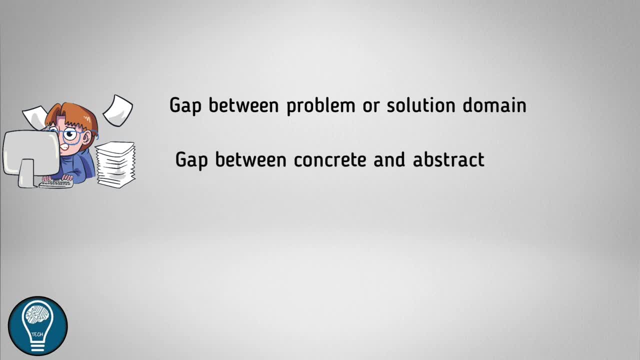 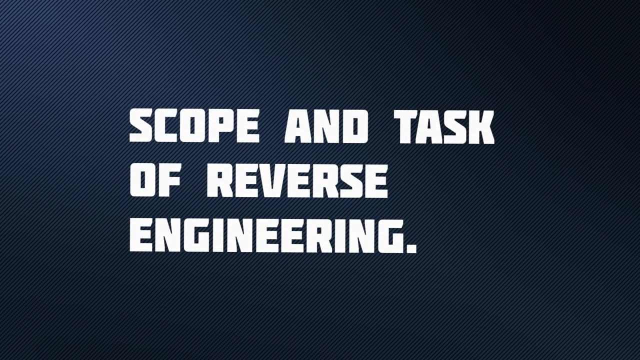 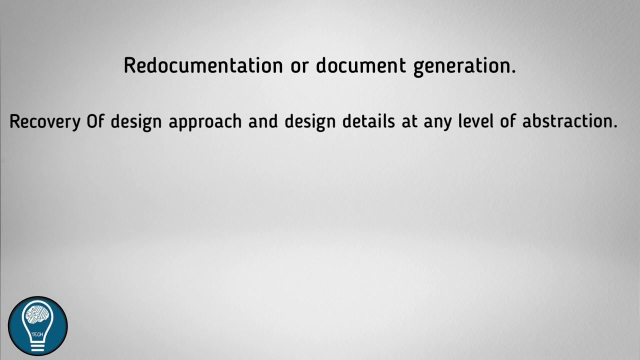 Gap between problem or solution domain. Gap between concrete and abstract. Gap between coherency or disintegration. Gap between hierarchical or associational Scope and task of reverse engineering, Redocumentation or document generation. Recovery of design approach and design details at any level of abstraction. 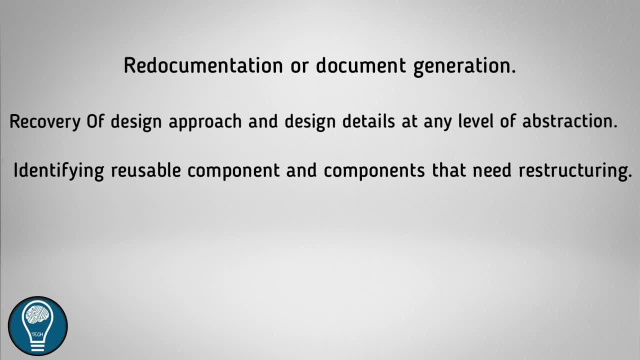 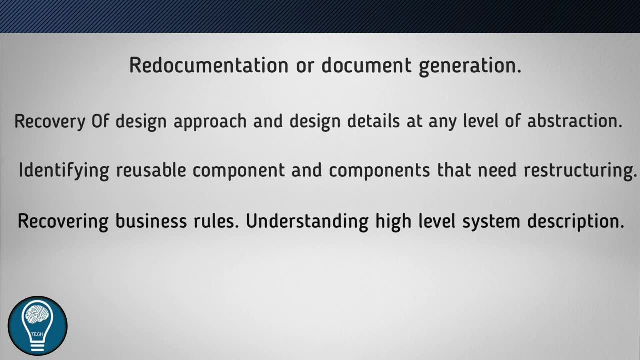 Identifying reusable component and components that need restructuring, Recovering business rules, Understanding high-level system descriptions, Understanding the environment And, furthermore, Providing a specific purpose for reverse engineering Approach and follow up on a specific theme: Toids- Goodbye. 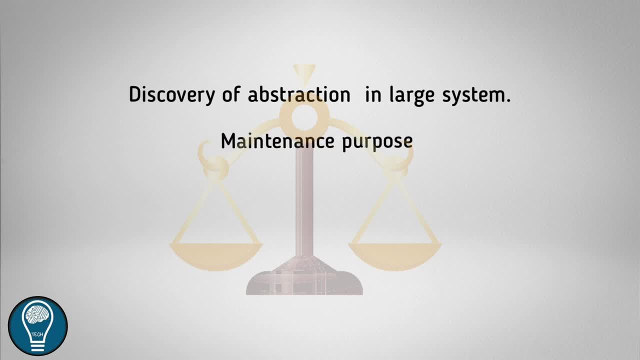 Next slide: Discovery of abstraction in large systems. Discovery of abstraction in large system: Maintenance purpose, Evolution purpose, Reengineering purpose, Levels of abstraction, Application, Application concepts, business rule, policies, Functions, Types of applications, Design and structure. 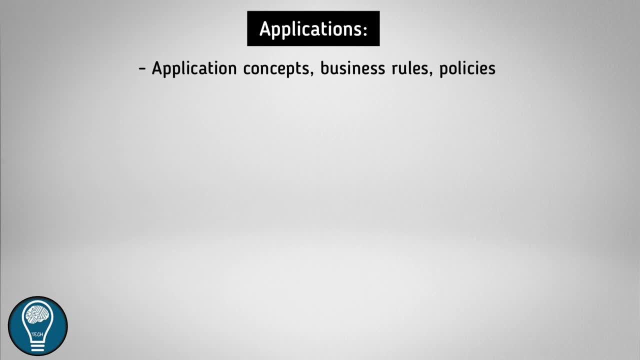 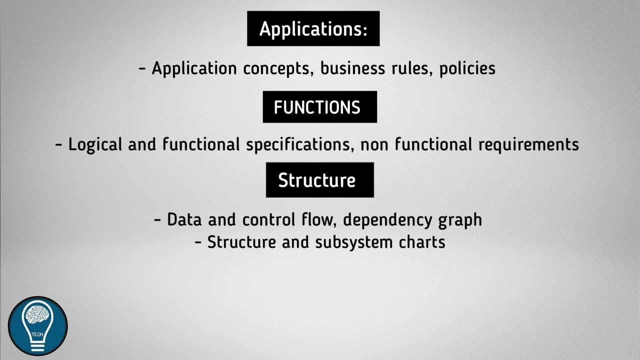 Data regulations. information, Problems of a system, Detail solution, Products, Underperformatives, Instruments, Logical and functional specification, non-functional requirement, Structure, Data and control flow, dependency graphs, Structure and subsystem charts, Architectures, Implementation Symbol tables, source text.